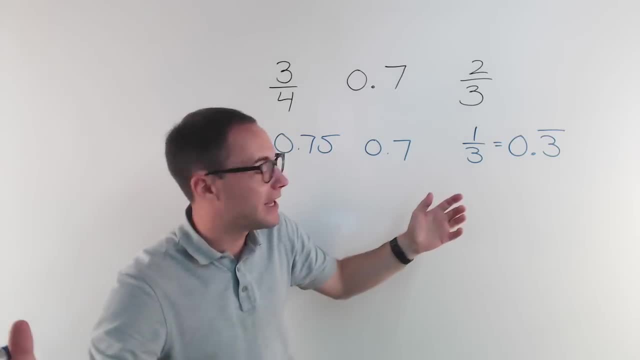 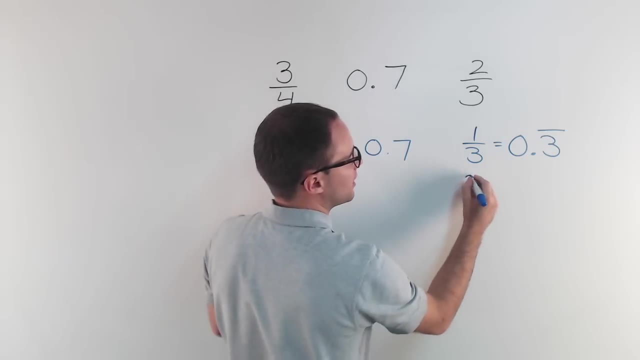 That number repeats That line means that number repeats That line means that number repeats. That digit repeats over and, over and over again an infinite amount of times. So 0.33333 forever. If that's 1 third, well then 2 thirds is just 0.6 repeating. 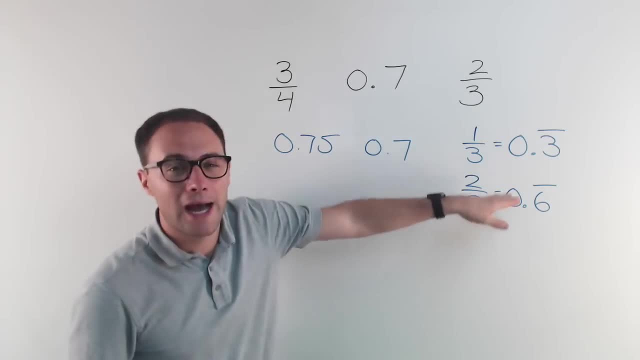 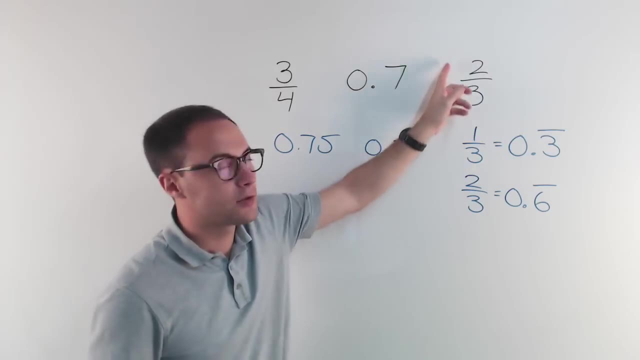 So 0.66666.. If you don't have those memorized, try to. They're going to help you out a lot. You'll see them all the time. But if not, you can always convert this to a decimal by dividing. 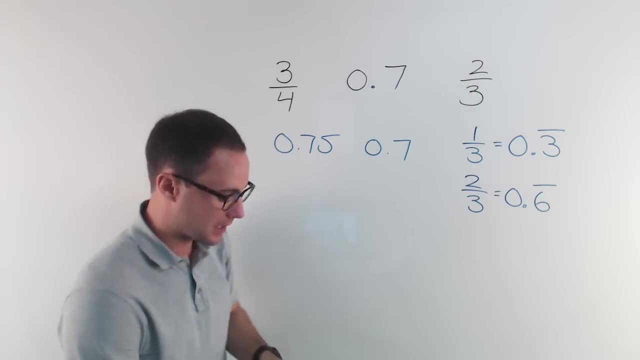 2 divided by 3, and you will get the same thing. Now that they're all decimals, hopefully it's pretty easy to see which one's greater or the greatest, and that is 0.75.. These both have 7 in the tenths place. but then we have to go to the next, and if I wanted 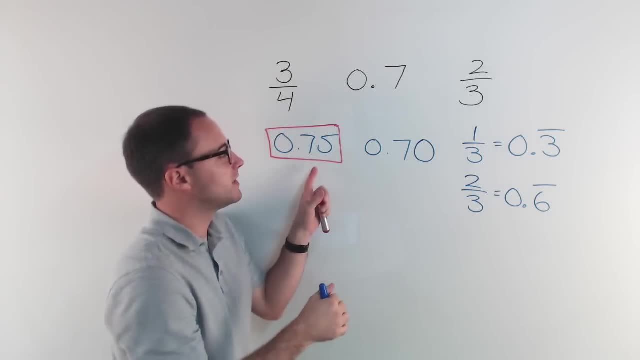 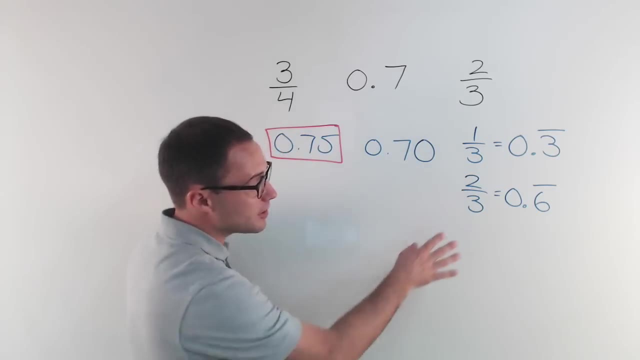 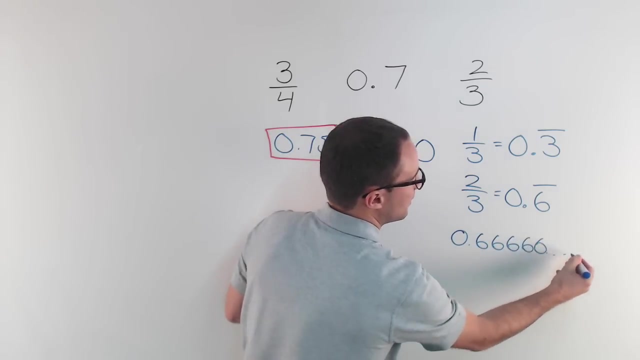 to. I could add a 0 there, So it's really 75 hundredths compared to 70 hundredths and obviously that is greater. And don't get confused: 0.6 repeating is like 0.66666 forever, but we don't care about all. 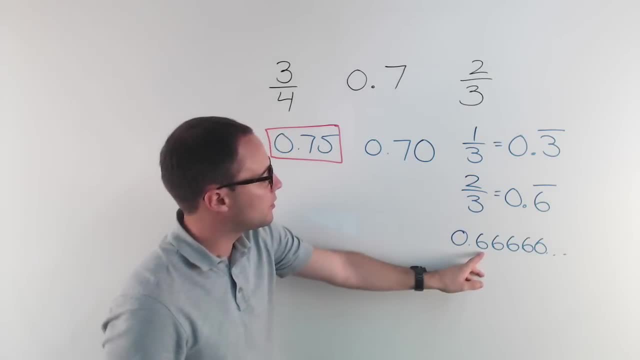 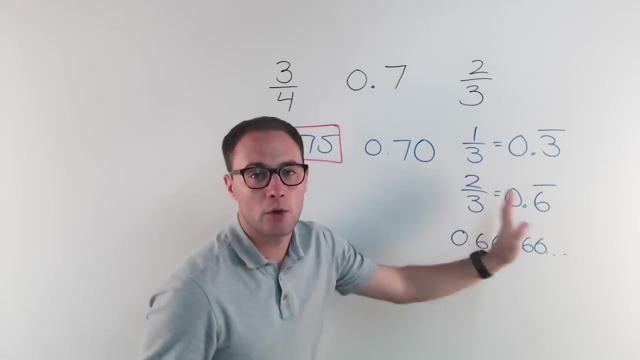 those sixes at the end or going to infinity. we're looking here right off the bat at the tenths place. 7 is greater than 10, so we don't even care what's after. We already know that that's actually the least. 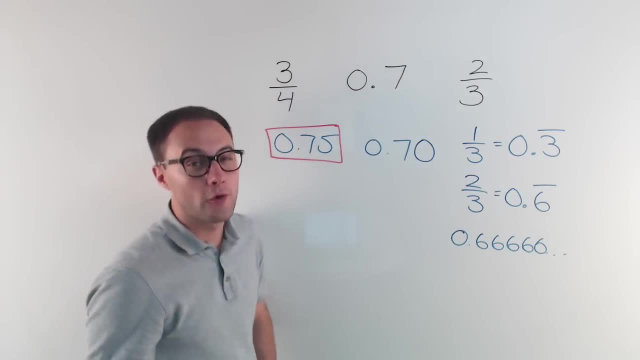 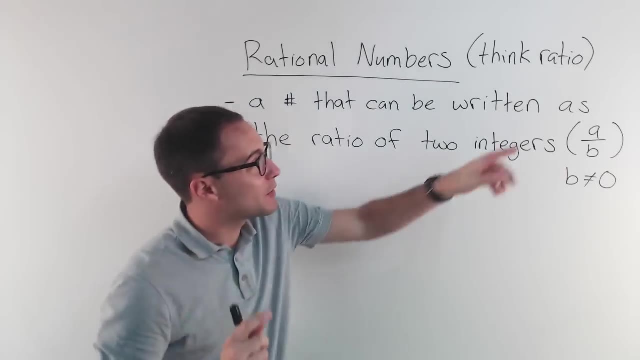 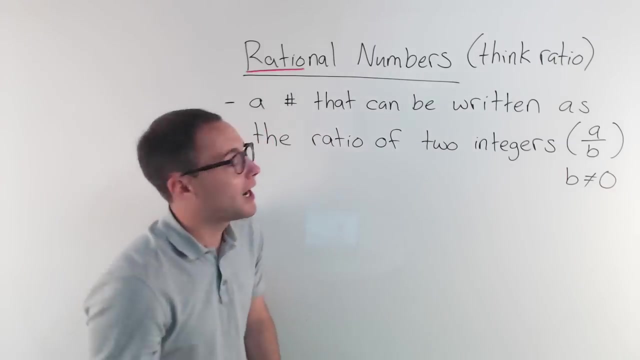 So, if you have the option, take 3 fourths of a cookie. Okay, Let's first talk about what are rational numbers. When you see rational numbers, think ratio. right, It's in the word rational. the first part is ratio. 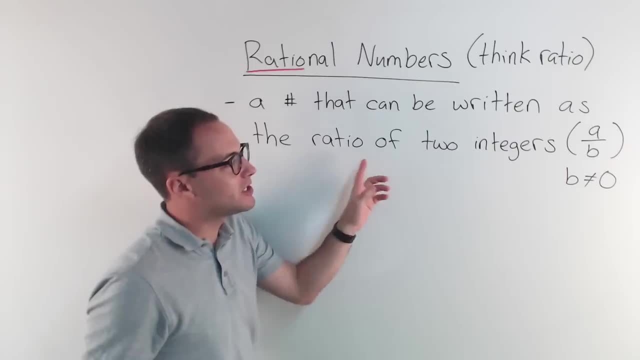 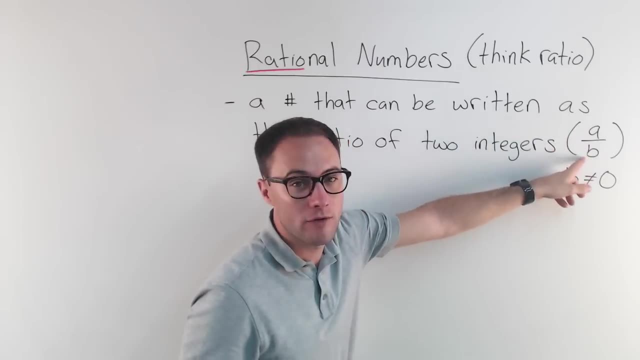 So rational numbers are just numbers that can be written as the ratio of two integers, So a ratio we could write like a fraction. right A to B can be written as A over B, as long as B is not 0, because, remember, if B is 0,. 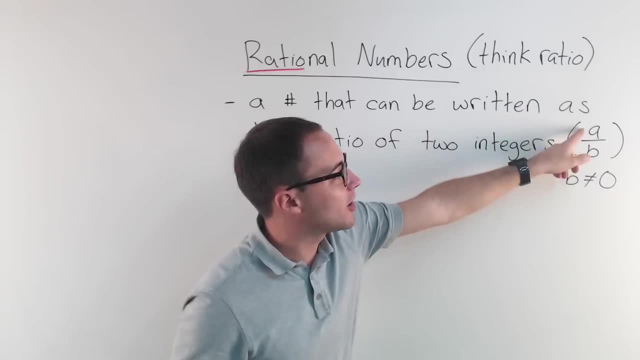 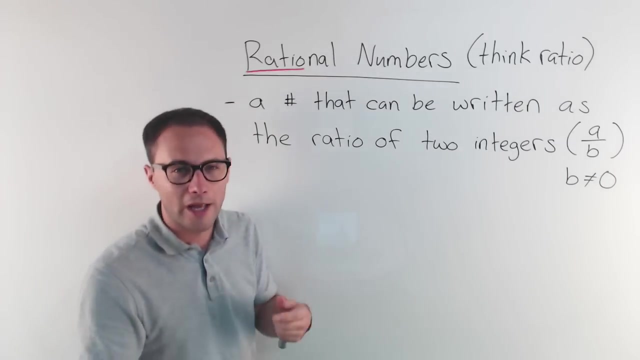 then that's undefined, right? So as long as A and B are integers, okay, then you're good. you've got rational numbers. Now we might be. you might be getting a little bit confused: talking integers, talking rational numbers, and you're thinking whole numbers and you're getting them all mixed up. 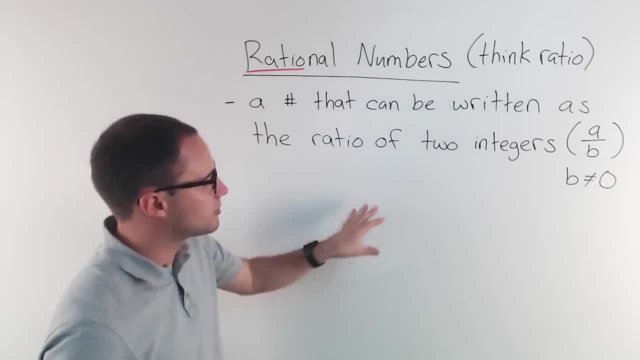 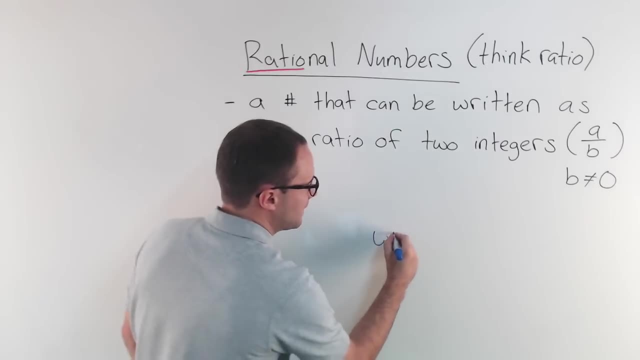 Well, let's just do a quick little, a little chart or a little graph here to help you remember what's what. Well, at the very basic, we have whole numbers, Okay. Okay, Whole numbers. All right, That's what you dealt with when you were a little kid, right? 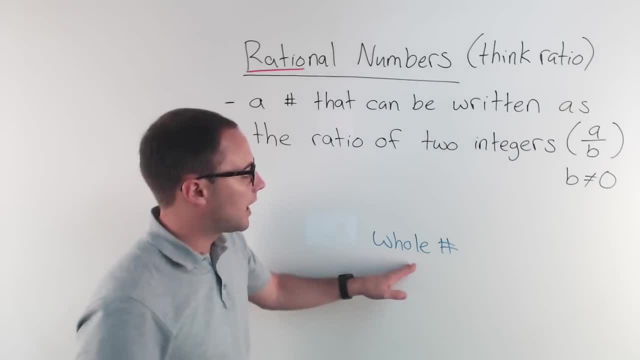 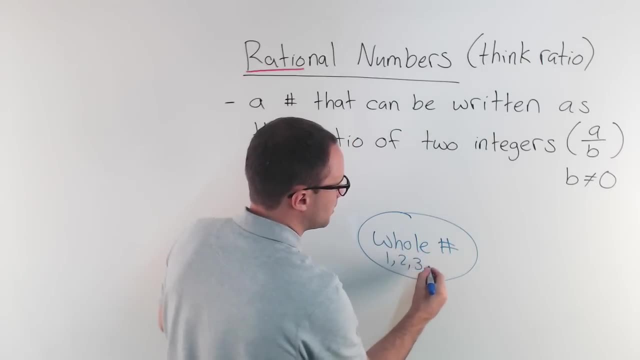 One, two, three, four, five, six, seven, eight. you know, keep going. No negative numbers here. Okay, No decimals, right, Just whole numbers: One, two, three, four. I'm sorry, I should have zero there. 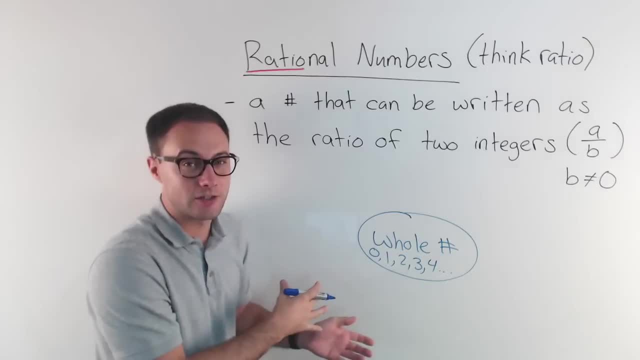 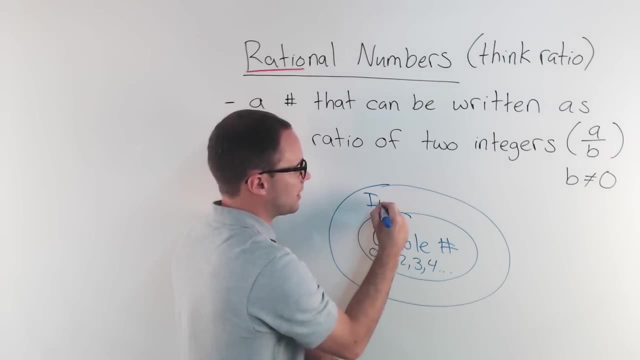 Keeps going forever. Then we talked about integers, right? Well, integers include all the whole numbers, but then it also includes- let me write that- but then it also includes the negative whole numbers. So then we've got negative one, negative, two negative, three negative four, and so on. 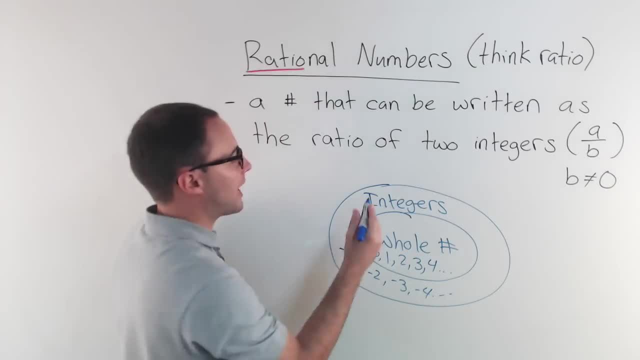 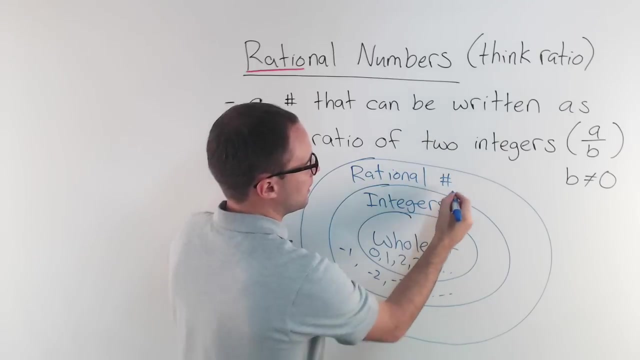 But it also has all those whole numbers still. Now we're getting into rational numbers. Now, rational numbers includes all the whole numbers. it includes all integers, but now we are also going to talk about rational numbers, Okay, Okay. So we're going to talk about fractions and decimals. 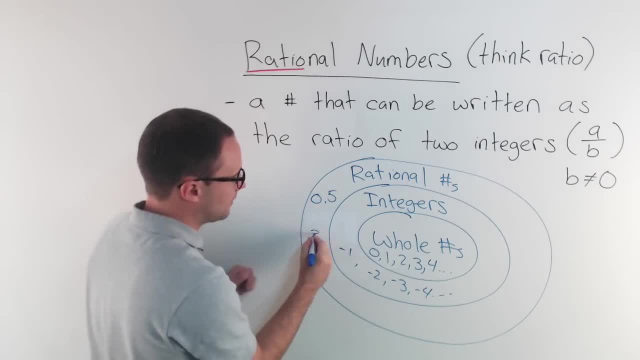 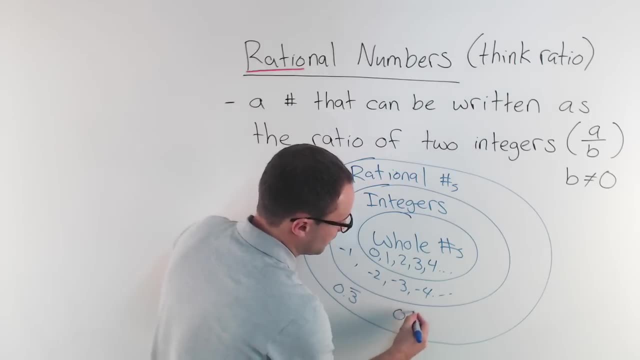 So now that's what we're talking about, rational numbers. So 0.534, 0.3, repeating let's see 0.78, negative two thirds right, Negative 4.5.. Those are all rational numbers, okay. 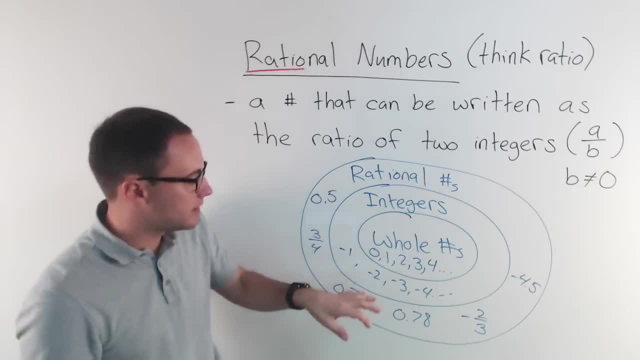 So that's important. Hopefully that helps kind of break it down for you the difference between whole numbers and rational numbers. Rational numbers include all of this stuff here. okay, So let's look at some examples of rational numbers and really go over this definition. 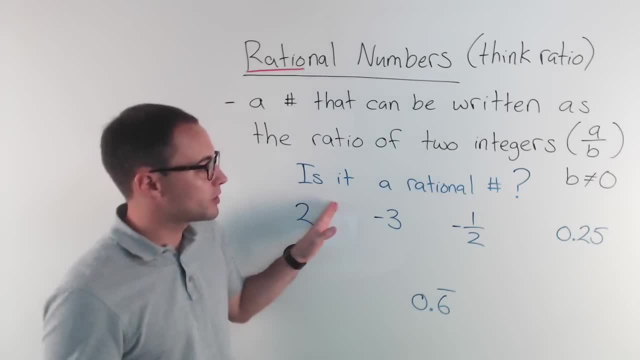 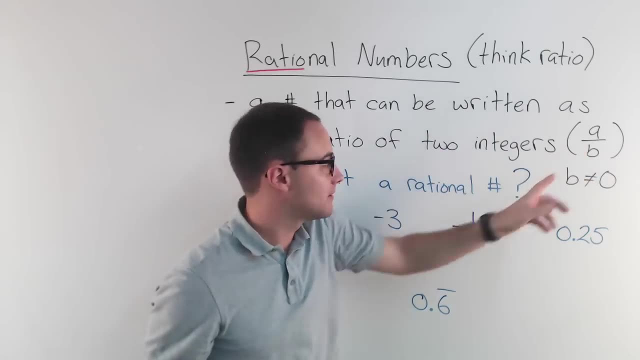 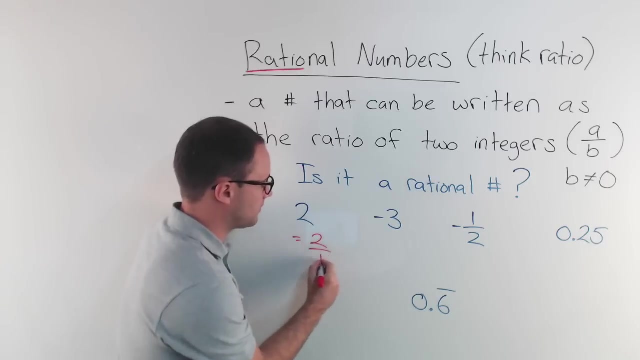 Okay, here's some examples. We're kind of testing: is it a rational number? So can we write it as a ratio of two integers where the denominator is not zero. So two, is that a rational number? Well, yeah, we can write that as two over one. 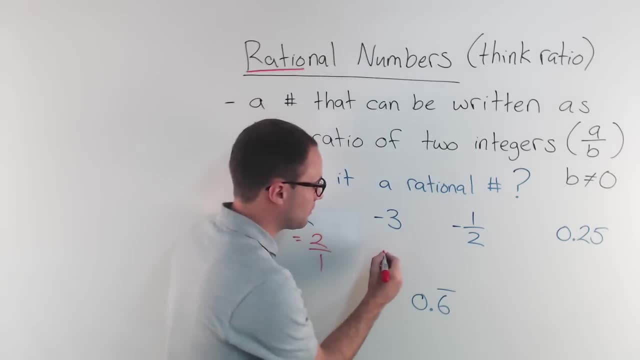 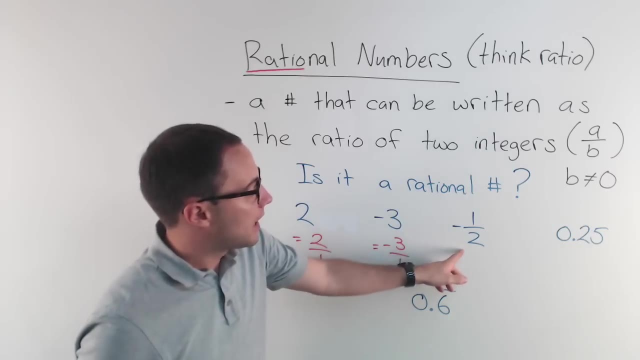 Two and one are both integers. We're good. Negative three can be written as negative three over one. Those are both integers. Remember: negative three is an integer, Negative a half. Well, I can write that as negative one over two. I can also write it as one over negative two. 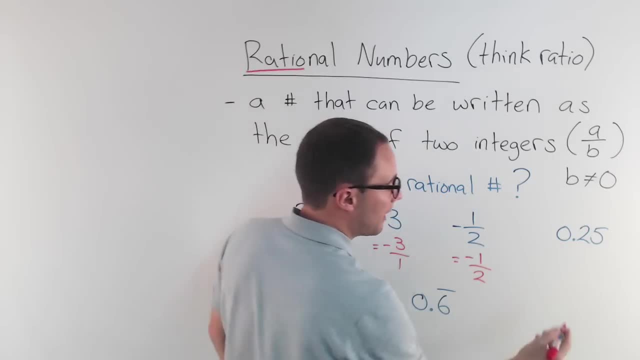 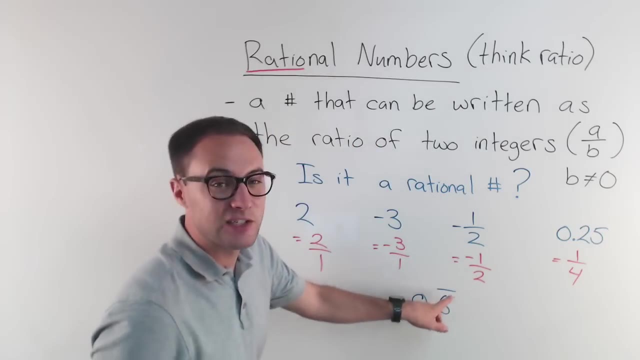 Those are both integers, so that's good. 0.25 is the same as one fourth, That's good, Those are both integers. 0.6, repeating If you remember from earlier, That's the same as two thirds. So again, those are both integers. 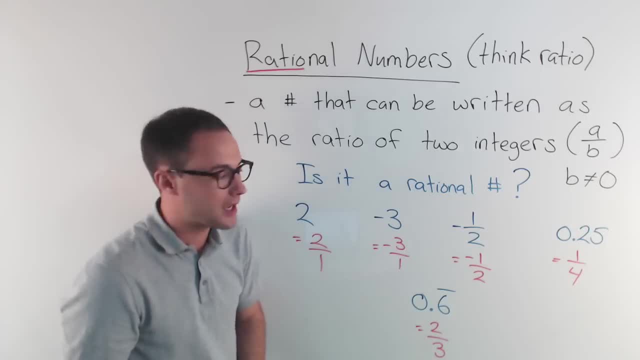 So all of these are examples of rational numbers. okay, An obvious example of a number that's not a rational number would be pi. right, Pi continues forever, never repeats, So you cannot write it as a ratio of two integers like a over b. 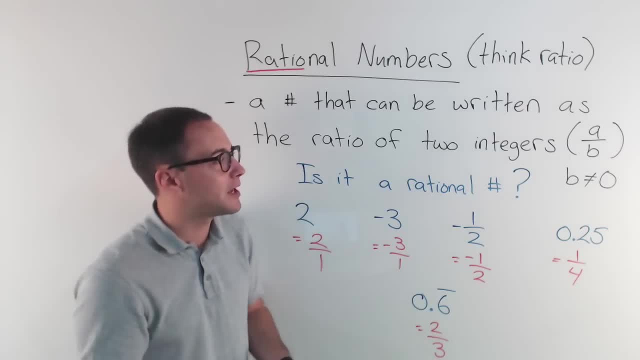 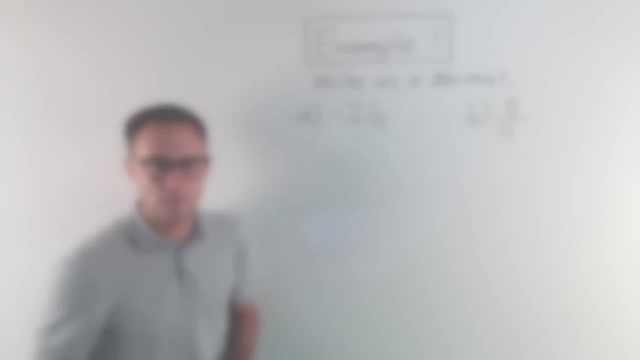 So pi is not rational, That's irrational. And there's other examples, But Here's some ones of rational numbers and that's how you check. Let's do an example. Okay, example one: Write as a decimal. So each of these we're going to convert to a decimal. 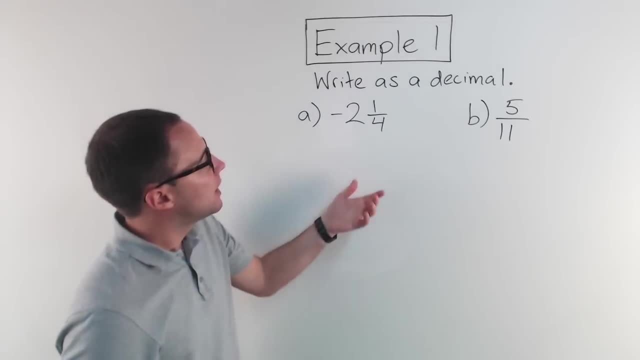 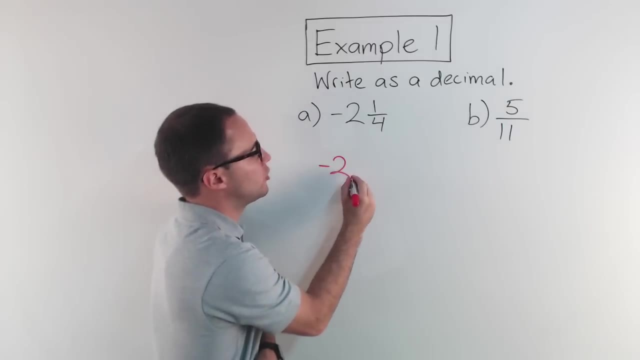 Fractions and decimals can go. you can go back and forth between the two Now negative two and one fourth. Well, I know that's two wholes. So that's going to be negative two. My decimal point is going to be there. And then I've got to think: well, what is one fourth as a decimal? 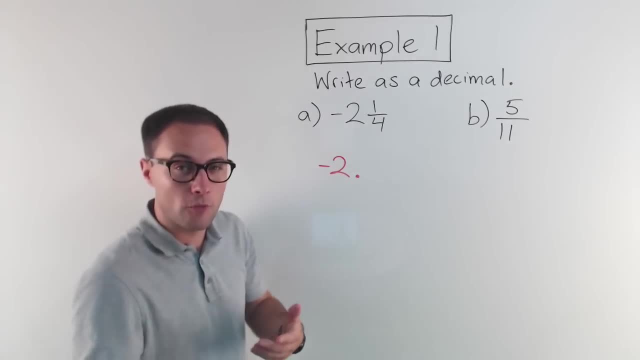 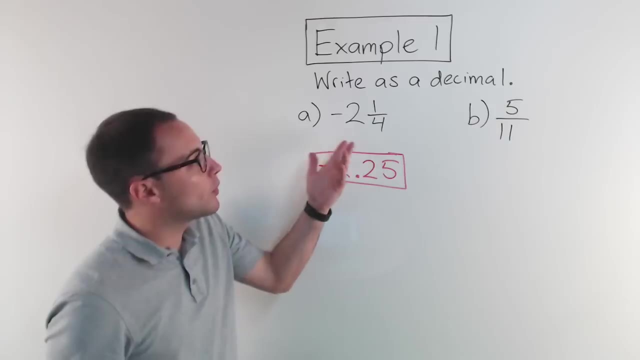 One fourth as a decimal. Okay, So my decimal is point two five. hopefully you have that memorized. So that's simply negative two point two five. Now another way to do it: if you wanted to, you can convert it to an improper fraction. 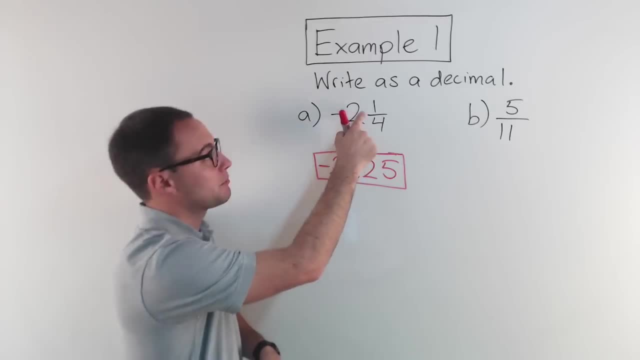 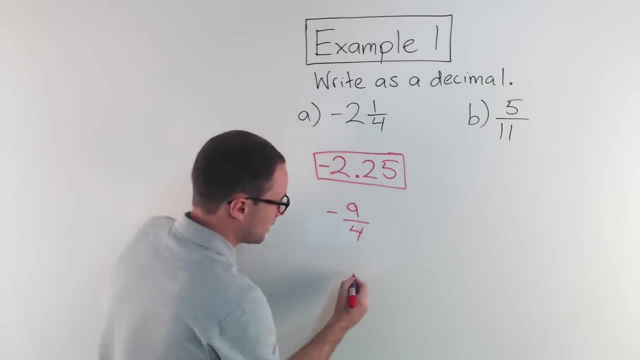 which would be right. four times two is eight plus one is nine, negative nine over four. And then this just means division. So I can do nine divided by four. well, that goes twice. Subtract That's eight, that's one. add a decimal point, add a zero. four into ten is two, again that's. 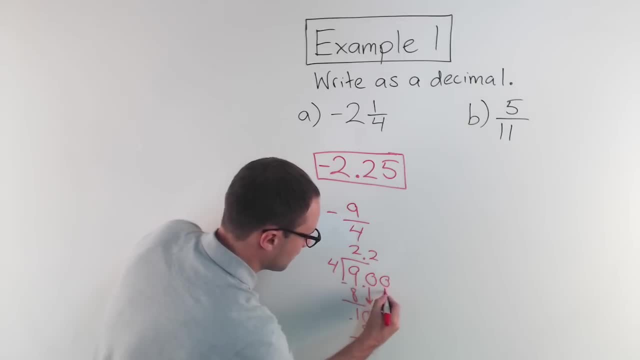 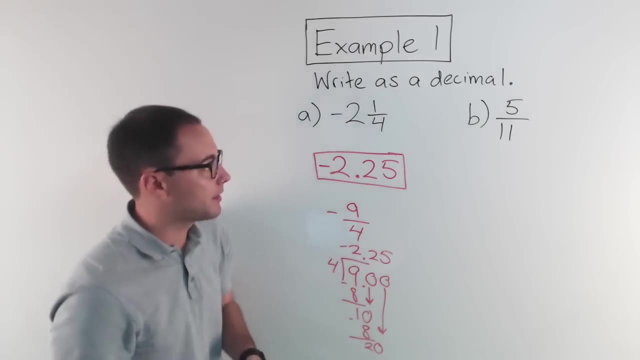 eight, subtract, I get two. bring another zero down. four to twenty is five, And remember it was negative, so negative. two point five, We get the same exact thing. Okay, Now let's look at the next one. Five elevenths. 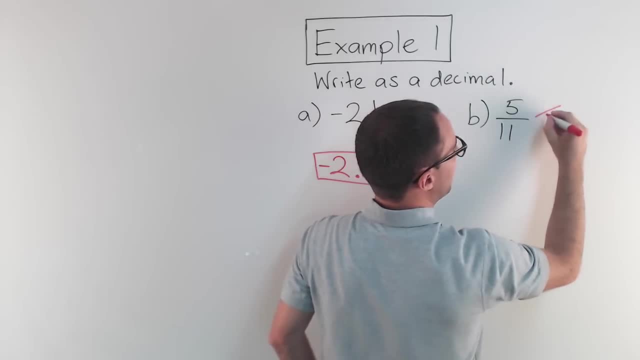 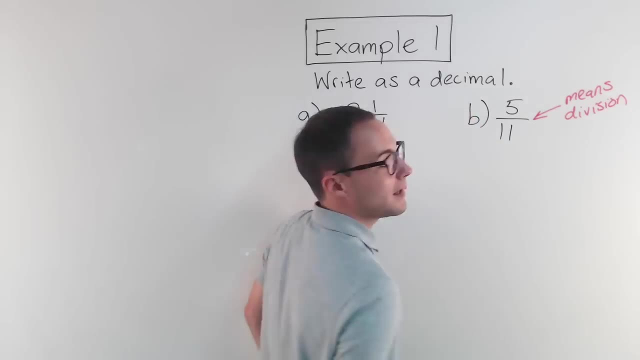 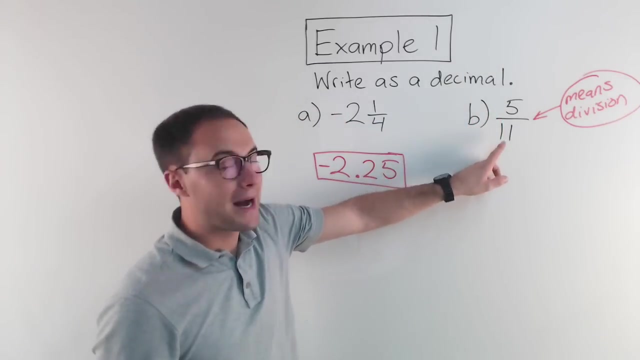 Again, like I just said this line: in a fraction that means division. okay, That's really important. Okay, I would definitely write that down. So this means five divided by eleven. So to convert it to a decimal, that's all we have to do. 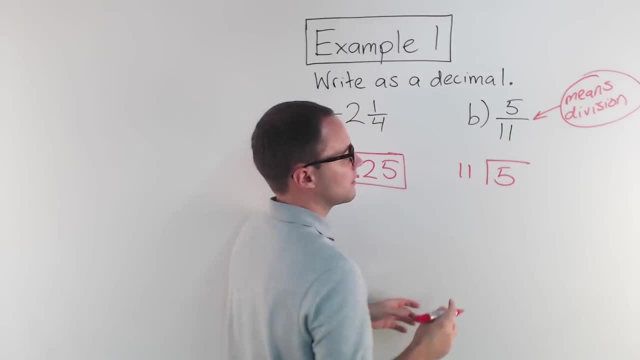 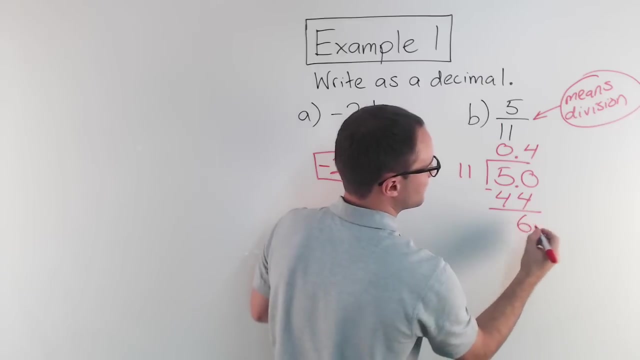 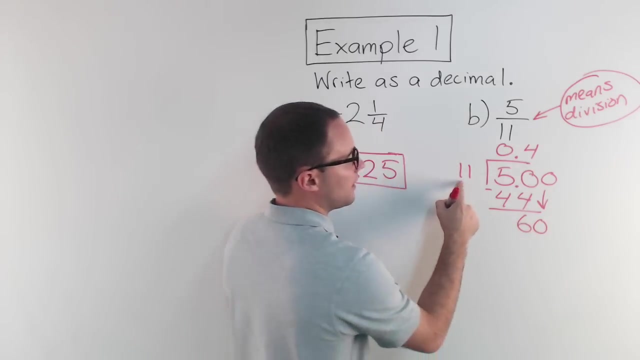 Five divided by eleven, Eleven into five, well, zero times. So I add a decimal here, add a decimal here, add a zero. Eleven into fifty goes four times, That's forty-four subtract, I get six. I'm not done. add another zero, bring it down and I get sixty. 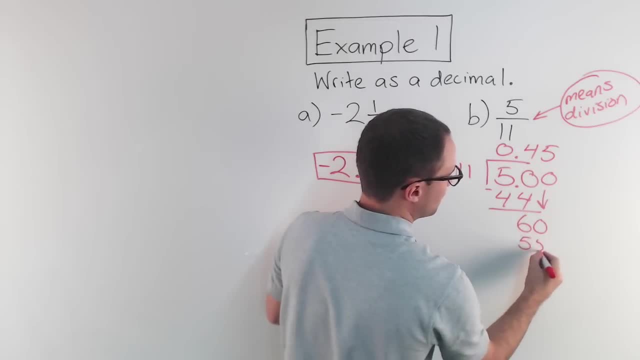 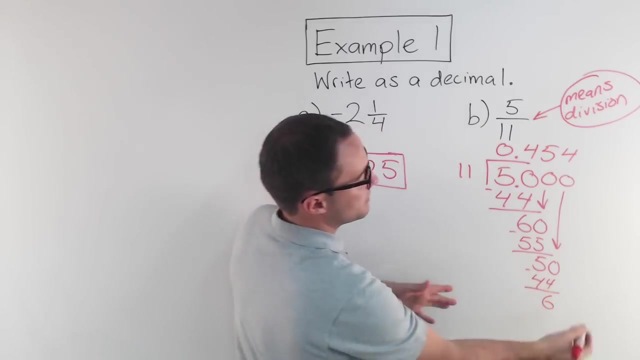 Eleven into sixty goes five times. that's fifty-five subtract, I get five. add a zero, bring it down fifty. Eleven into fifty is four and you might start to notice a pattern. right, That's forty-four subtract, I get six. it would be sixty again, so four-five again. 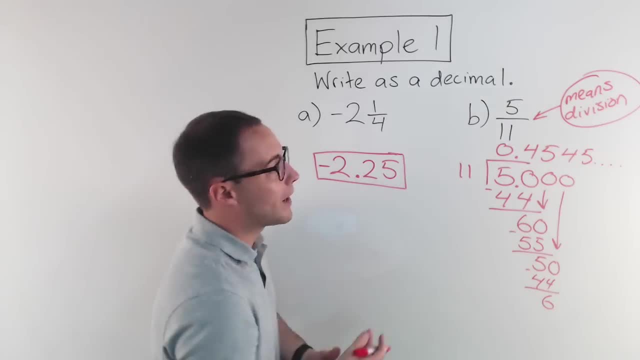 and it's going to keep going on forever. So the way that I write this as a decimal, since the four and the five are repeating, I'm going to write it as zero point four-five, with the line over the four and the five. 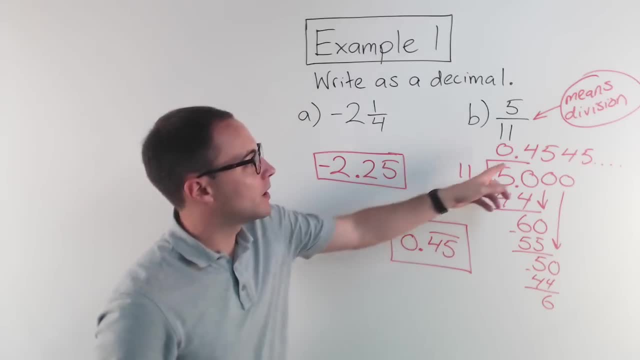 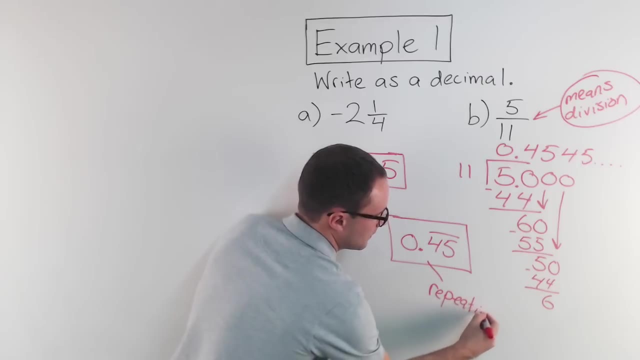 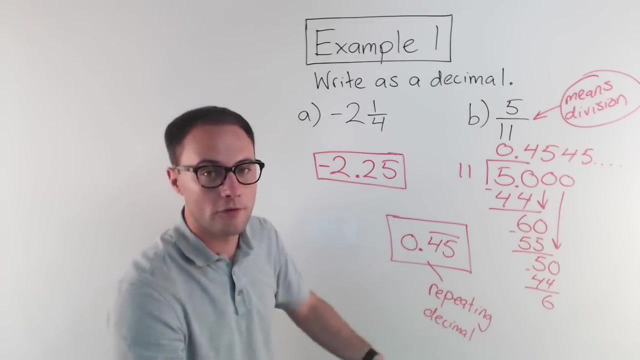 That means The four and the five are what's repeating. okay, This is called a repeating decimal. okay, because the four and the five repeat over and over and over again: Zero point four-five, four-five, four-five, four-five right. 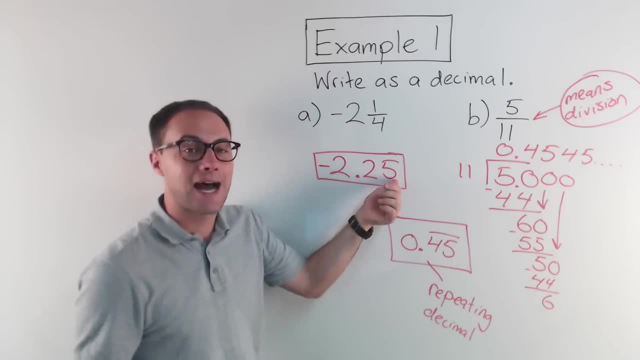 On and on and on This one. it's not repeating, it's stopped, it ended, So we call that. you can think of the movie The Terminator. It's called a terminating decimal, So make sure you know the difference between the two. 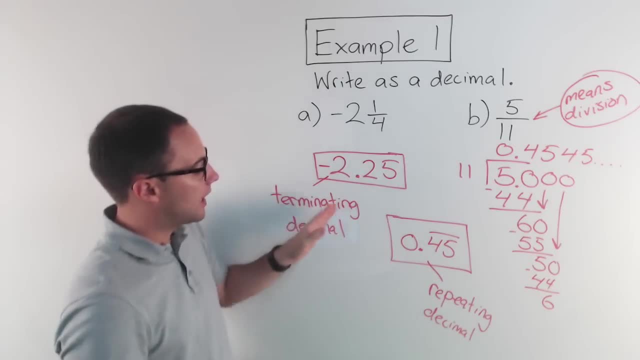 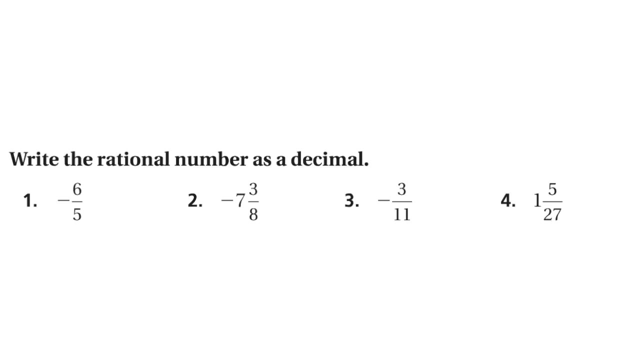 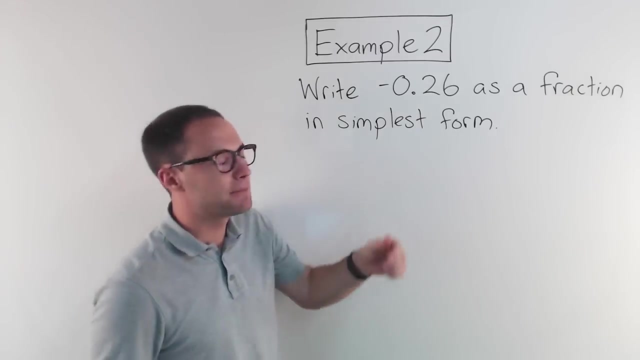 Terminating decimals. they stop, they end, they terminate. Repeating decimals: repeat On and on and on forever. okay, Here's some to try on your own, All right. example two: Write negative zero, point two-six as a fraction, in simplest form. 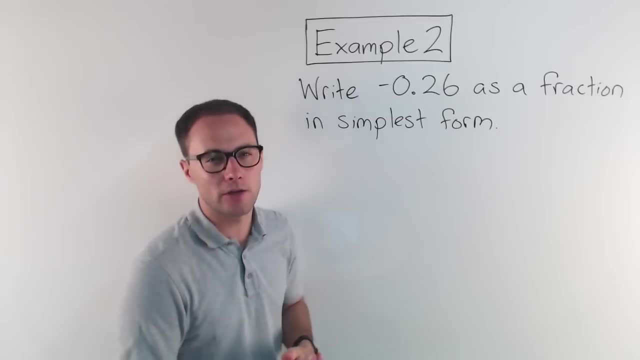 Well, to be able to do that, you need to know your place values. So negative two point six: I'm going to. Obviously my fraction is going to be negative, so I'm not going to worry about that yet. I'll just kind of put that there and kind of forget about it a little bit and just concentrate. 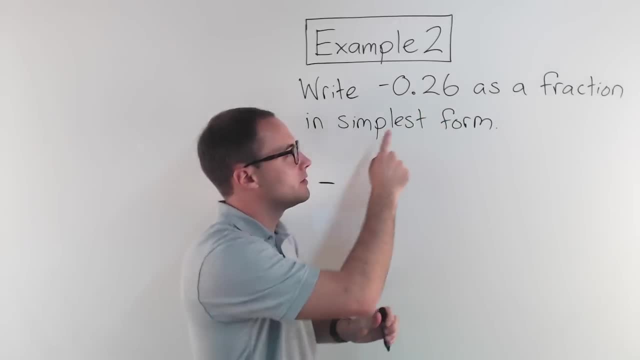 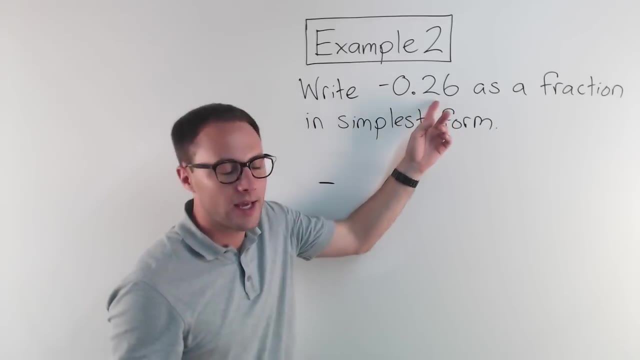 on this Zero point two-six. Well, if you know your place values, this is the tenths place, That's the hundreds place. So if you read it out loud, If you read it out loud to yourself, and you can say twenty-six hundredths, that gives. 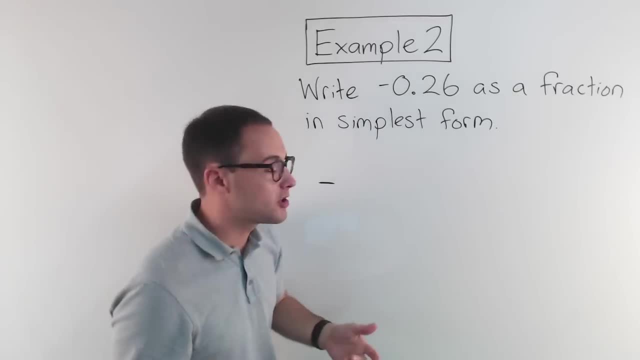 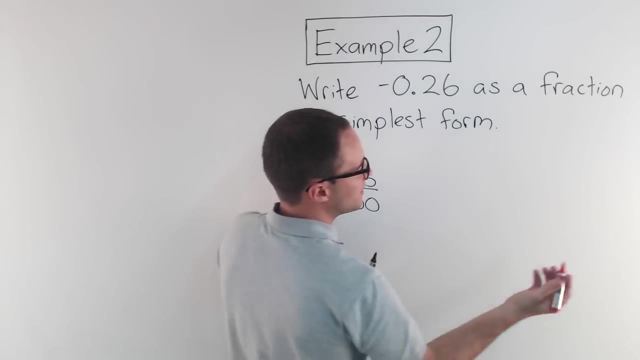 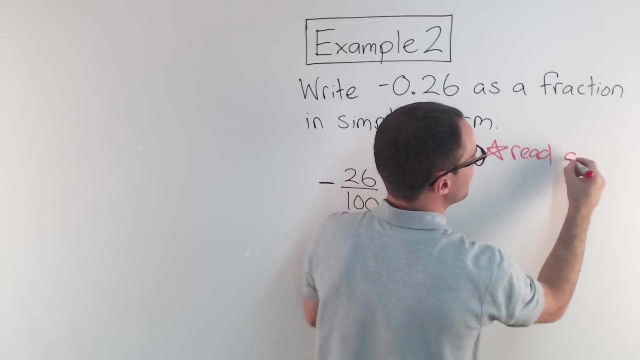 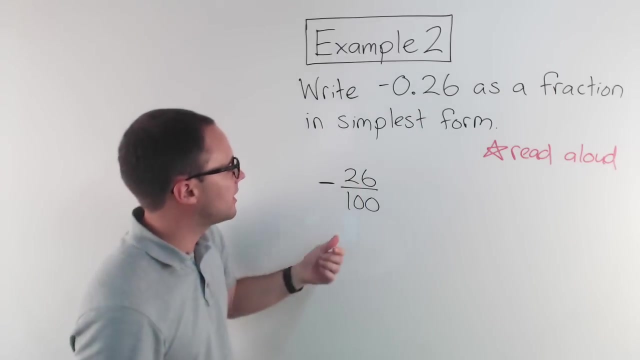 you kind of a hint as to what the fraction is going to look like. Twenty-six hundredths, okay. So maybe write yourself a little hint When you're converting it from decimals to fractions. read it aloud, Use those place values And that will give you an idea of what it's going to look like as a fraction. 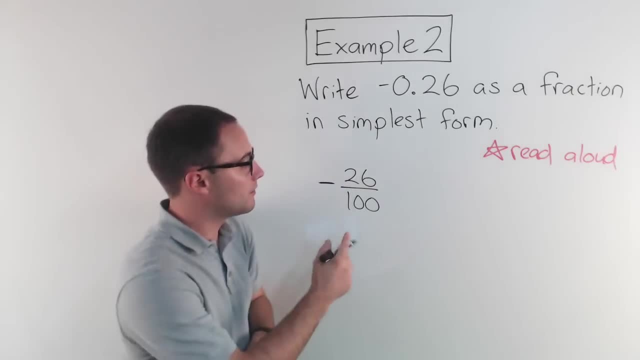 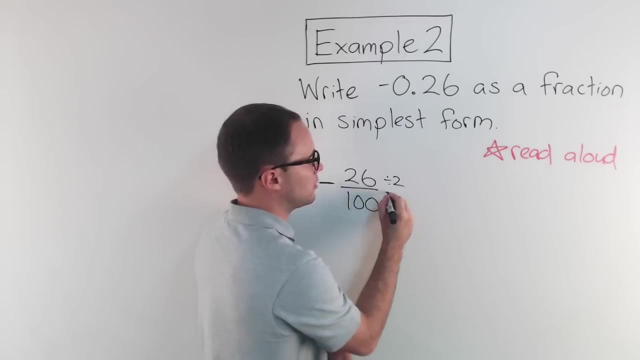 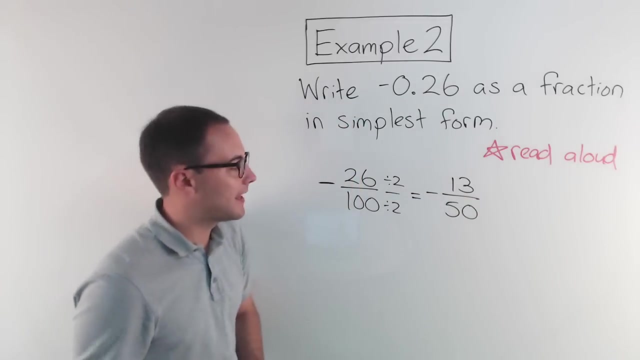 Now the second part. make sure it's in simplest form. Well, this is definitely not in simplest form. They're both even numbers, So I can divide that by two and divide that by two And I get negative thirteen over fifty. 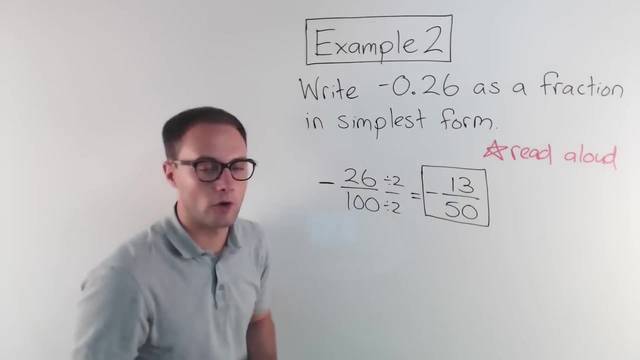 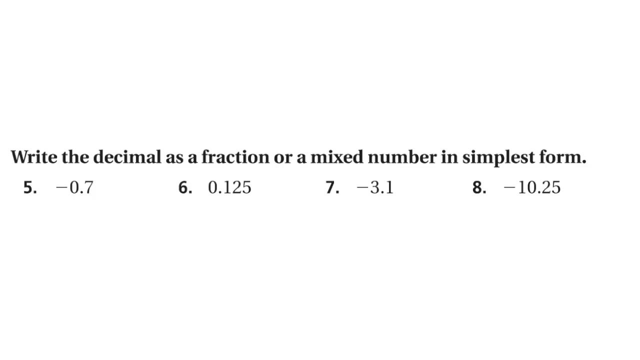 And that is now in simplest form. So that's how you convert from decimals to fractions. Remember- just read it out loud- Remember your place values and simplify it at the end. okay, Here's some more to try on your own. 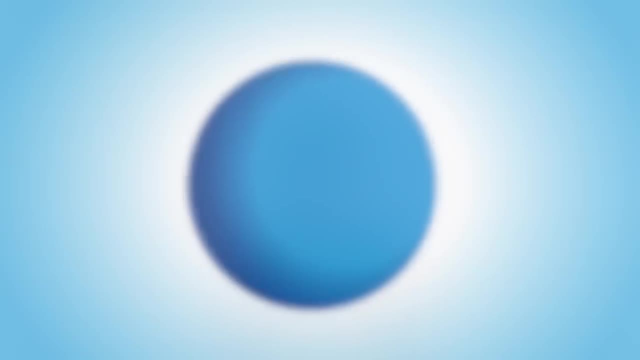 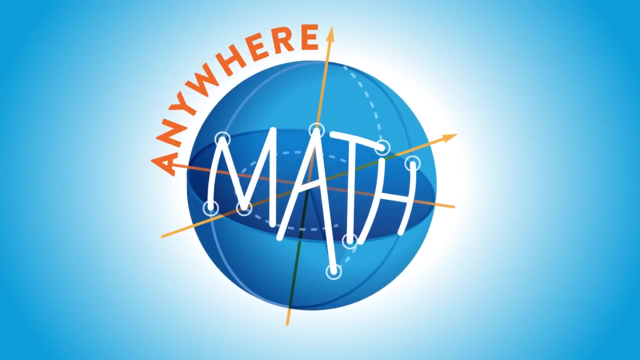 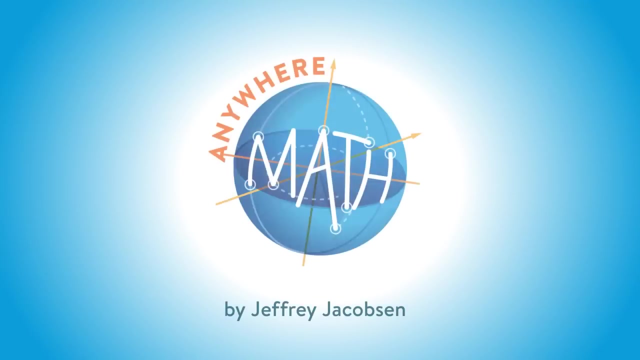 Thank you for watching And, as always, if you like this video, please subscribe And I'll see you in the next one.